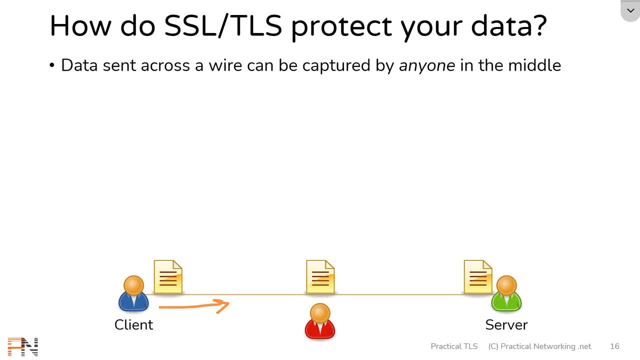 capture of data. Once data is on the wire, it is in somebody else's hands. Instead, the purpose of SSL and TLS are to protect what can be captured on the wire, And it'll do so in three ways. First, it'll provide confidentiality to that data. Confidentiality means that the data should 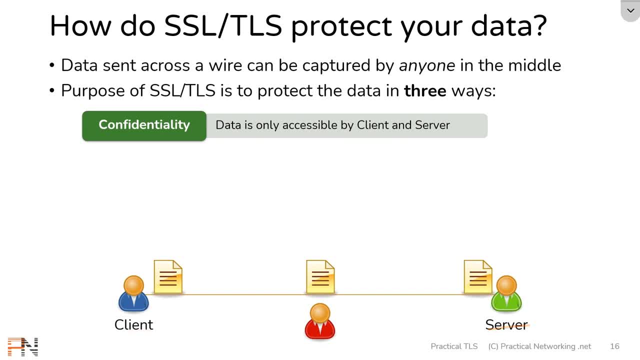 only be accessible by the client and the server Meaning on the wire. it should be encrypted So if someone in the middle captures it, they won't be able to make sense of what they captured. Next, SSL and TLS are going to provide integrity to that data, And what? 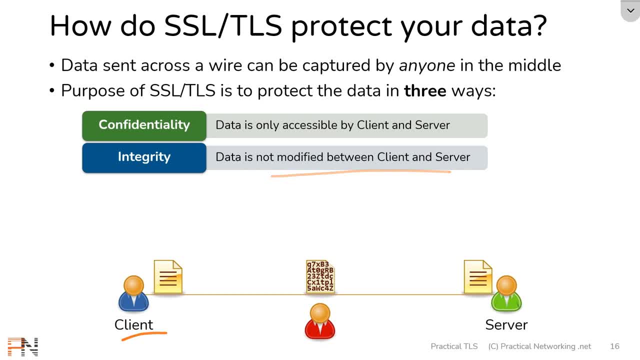 that does is it makes it so the data cannot be modified between the client and the server. Now to be clear, it doesn't actually prevent the modification of data, but it does enable detection if the data was modified. It's one thing to not be able to. 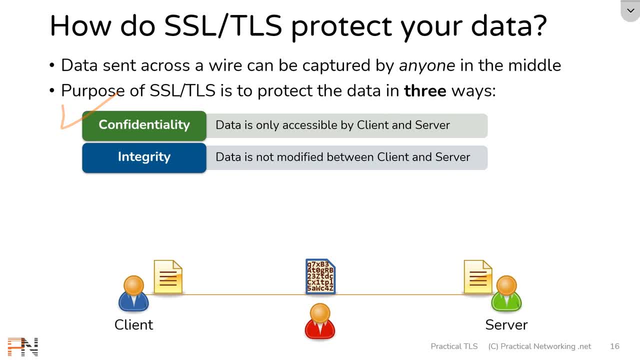 understand what is sent on the wire because of confidentiality, But it's another thing entirely to not be able to change what was sent on the wire With integrity. if this red user modifies some of the text in this message, the green user will be able to detect it and know that that message has been tampered with. 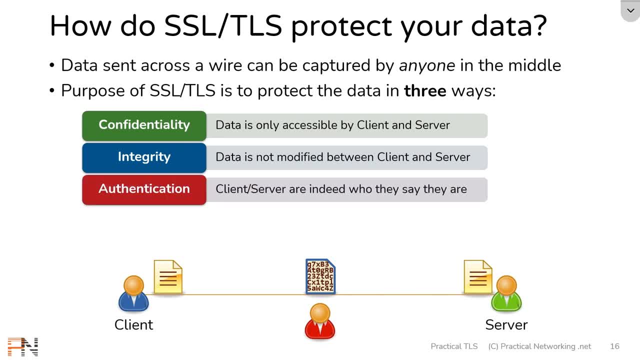 Finally, the last thing that SSL and TLS will do to data is going to validate the authentication of that data Meaning. they're going to make sure that the client and the server are indeed who they say they are. SSL and TLS will do this by validating the. 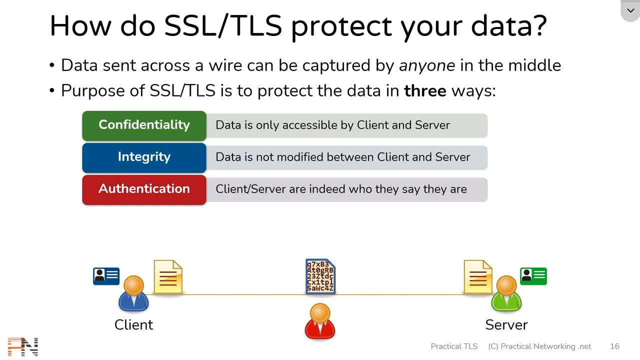 requests of the two parties in communication. So these three items are the main purposes of SSL and TLS, And each of these are provided via different cryptographic functions: Confidentiality is provided via encryption, integrity is provided via hashing and authentication is provided via the public key infrastructure. 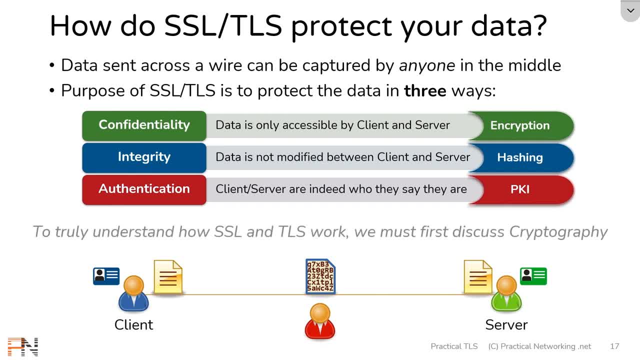 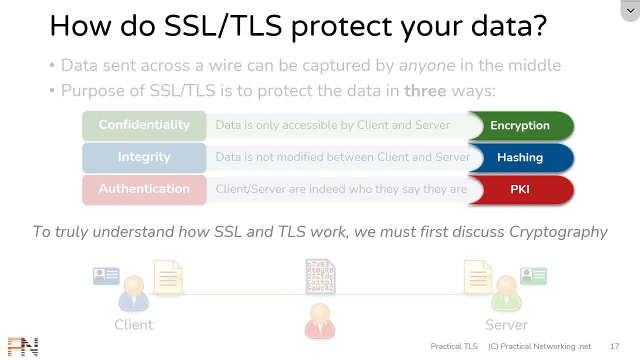 And to truly understand SSL and TLS, we must first discuss the cryptographic tools which make SSL and TLS possible. Subtitles by the Amaraorg community. In the next module, we'll be picking apart encryption, hashing and the public key infrastructure and showing you how those tools will provide confidentiality, integrity and 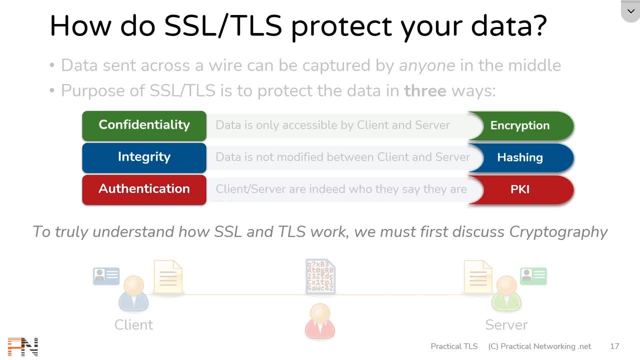 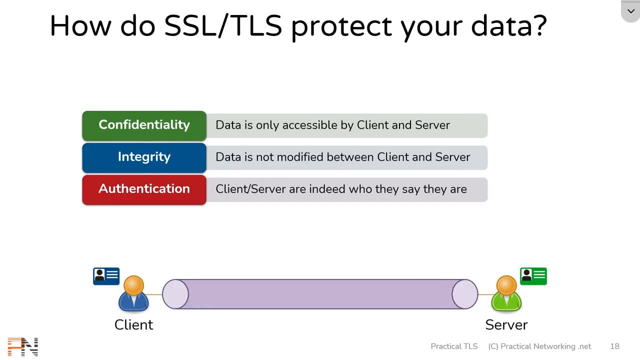 authentication. Before I close this lesson, there is one more idea I want to leave you with Notice. at no point in our discussion did we mention that there was a tunnel between the client and the server. You see, the idea behind an SSL tunnel is merely conceptual. 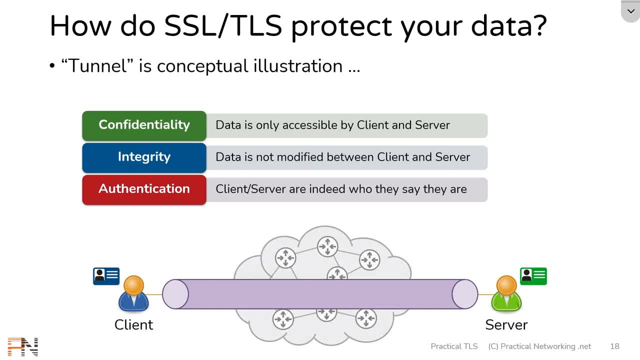 In reality, an actual tunnel is not literally built across the internet. It's simply a way to visualize what SSL and TLS are doing. To be clear, it is a useful visualization. In fact, it is one we'll use again throughout this course. 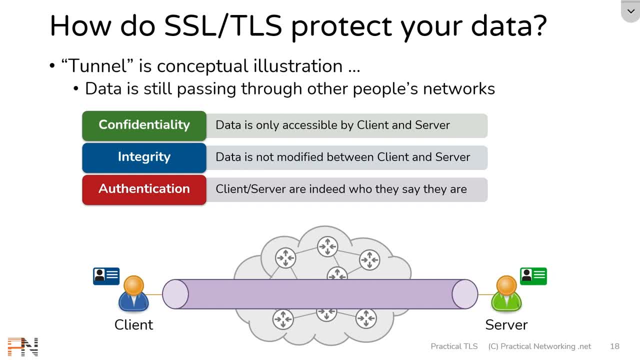 But in reality, the data you put on the wire is still passing through someone else's network. The only difference is with SSL and TLS. the data will be protected using confidentiality, integrity and authentication, Meaning if someone doesn't have a network, they won't be able to use it. 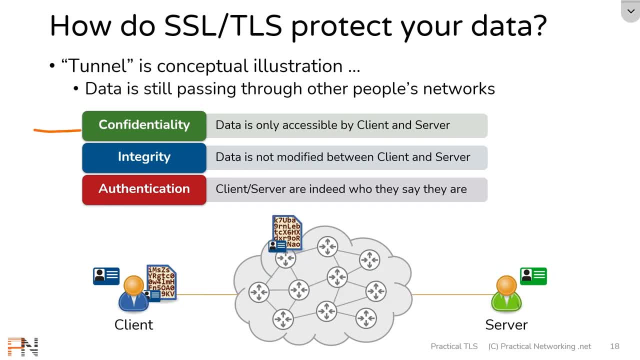 If someone does capture your data, they won't be able to read it because of confidentiality, they won't be able to modify it because of integrity, and they won't be able to pretend to be you because of authentication. That is what SSL and TLS are doing. 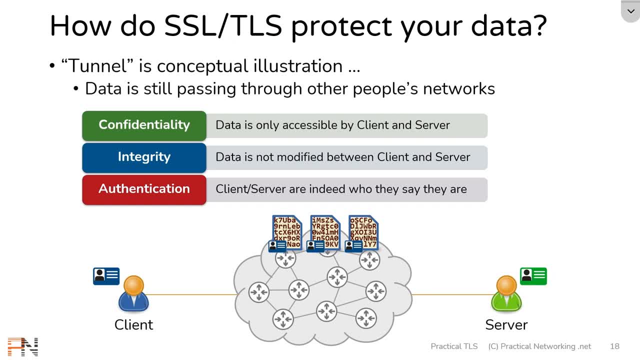 And, with that said, we bring this lesson to a close. The main takeaway is understanding the terms confidentiality, integrity and authentication. We'll be using these terms again and again throughout this course, so it's very important to have a very clear understanding of the terms. 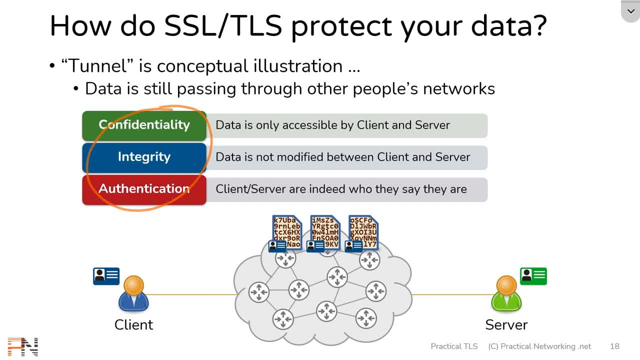 What each of them are and why you need all three of them in order to consider data sent across a wire as secure. In the next lesson, we'll describe two other terms that are often described, along with confidentiality, integrity and authentication, But that's it for this lesson. 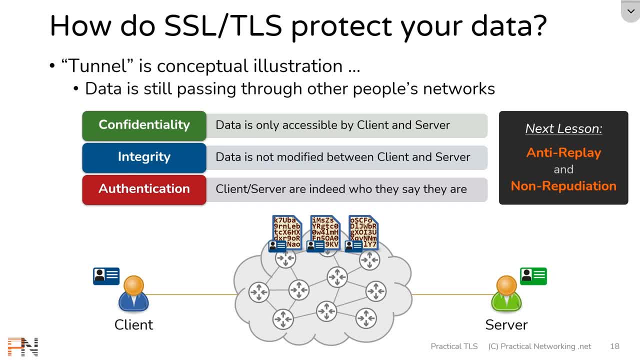 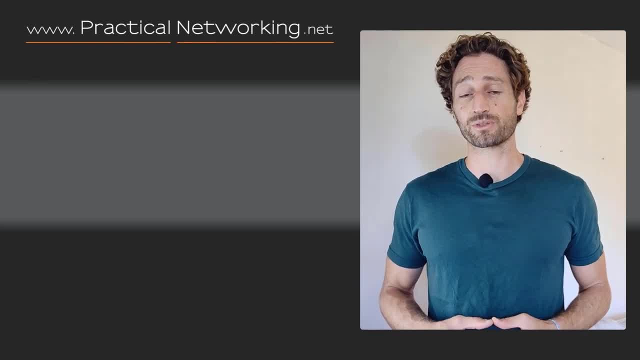 I hope you enjoyed this video. I want to thank you for watching and we'll see you in the next one. Did you enjoy this lesson? Do you want to understand the rest of the SSL and TLS ecosystem? If so, you'll want to check out my new course Practical Tools. 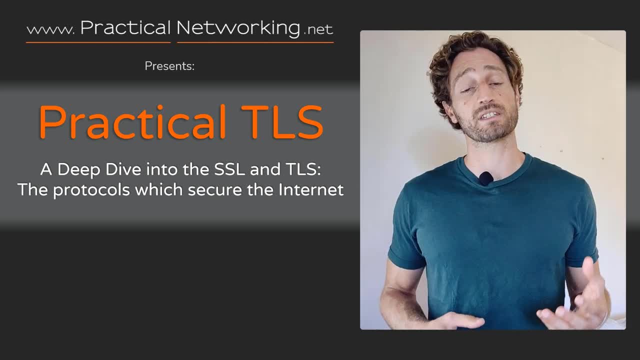 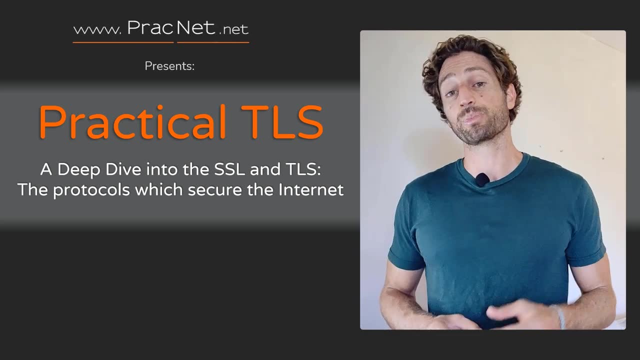 It's a comprehensive, deep dive into the world of SSL and TLS, designed to make you an SSL expert, regardless of where you are now. This course is all you need to help you become the next SSL expert on your team or to help 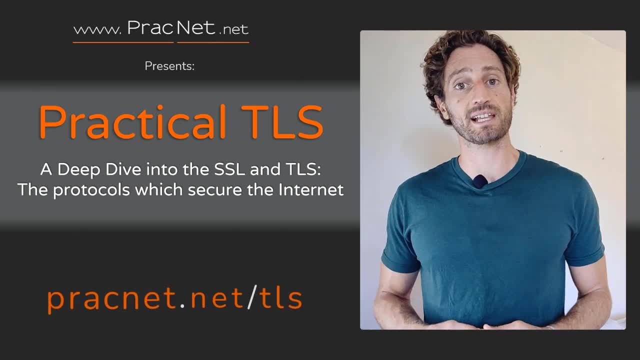 you nail those job interview questions. To learn more, check out pracnetnet, slash, TLS or click the link in the description. Otherwise, thank you for watching and we'll see you in the next video.